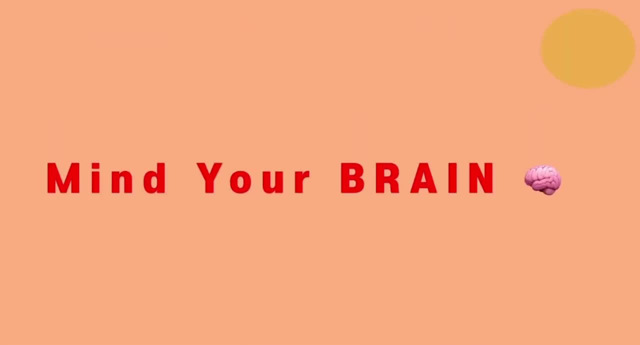 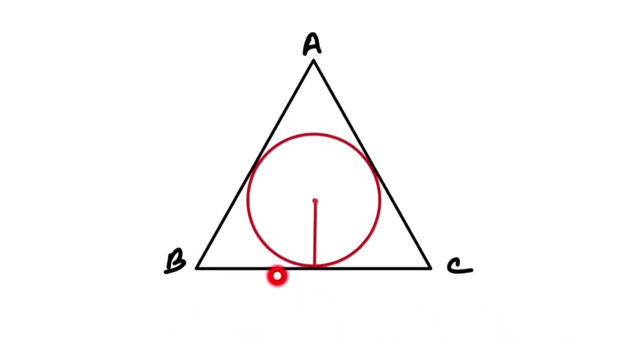 Hello everyone and welcome back. In this video we are going to solve this question. So sides of the triangle is given, BC is equal to 3,, AB is equal to 4 and AC is equal to 5.. And the area of the triangle is 6 unit. So you have to find the radius of the circle. This 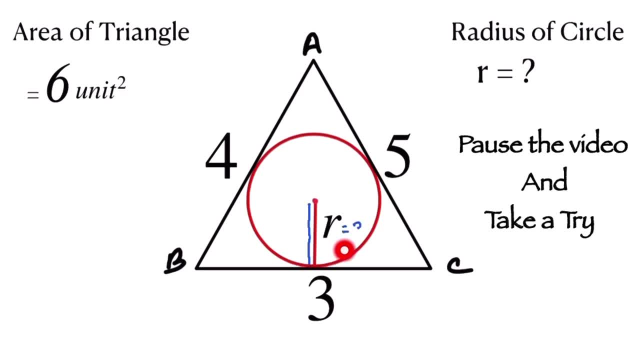 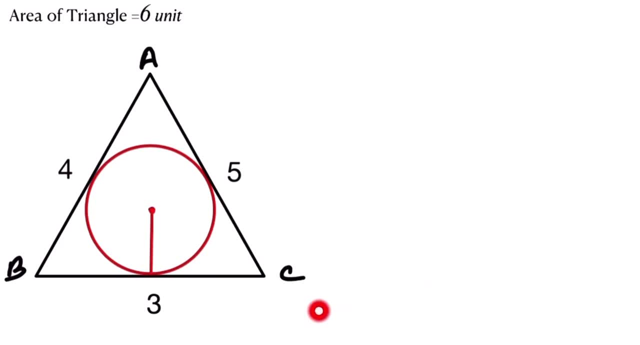 is 1.. So can you find this? If you can, then pause the video and take a try, Let's see the solution. So here, at first, we know that this is the radius of a circle that inserted inside a triangle Here OM form 90 degree on the base BC. So at first we join all. 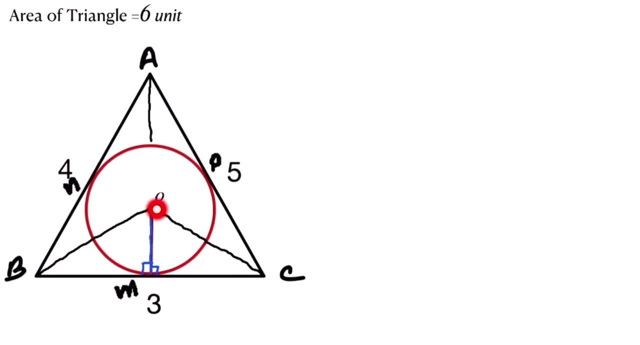 OB, OC and OA. So here OM is a perpendicular. So this is height, and here OP is also a height of the triangle AOC And ON is also the height of the triangle AOB. So here we form: there are total 3 triangle. 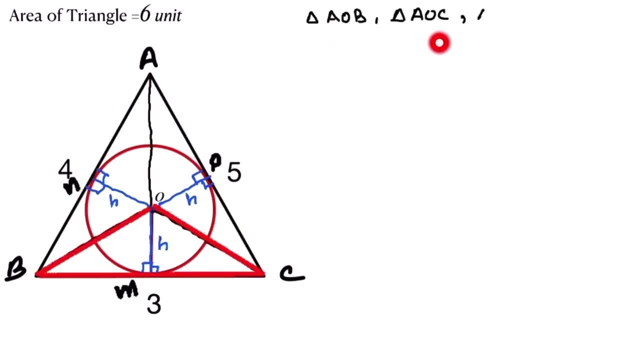 Triangle AOB, Triangle AOC and triangle BOC. So in the figure the radius is equal to height of the triangle. just look at here, om op and on all are the radius and this is also a height of the triangle. so area of the triangles is area of the triangle is equal to 1 by 2 base into height. 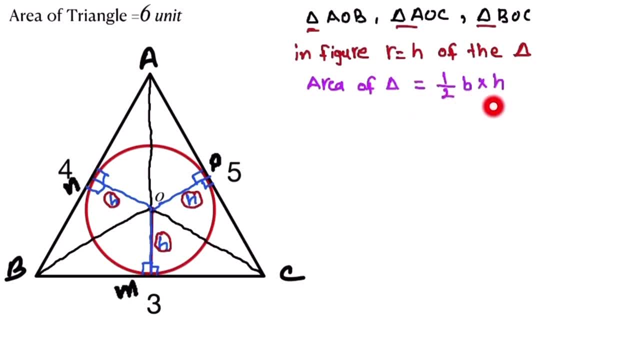 we know that at first- here name this all sides- bc is equal to a, sb is equal to b and s is equal to c. so now we take at first in triangle a or b, 1 by 2, and base is equal to a. so here we put a. 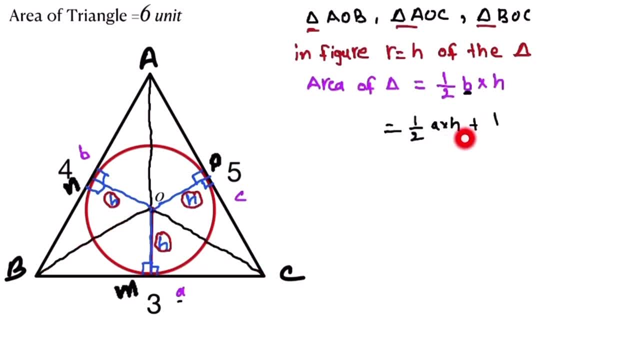 into h plus 1 by 2 and base is equal to. in triangle a or c, b into h plus 1 by 2, and in triangle b or c, height is equal to h and base is equal to c. so here we look: 1 by 2 and h is common.